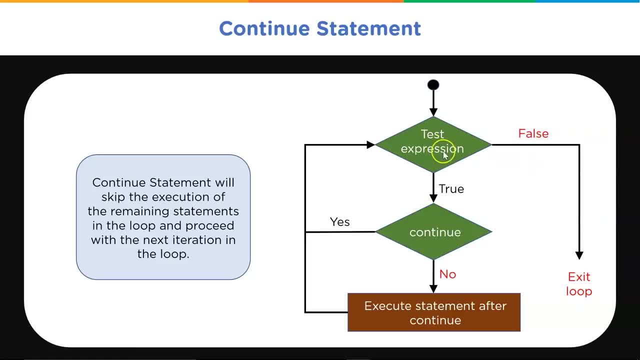 So the test expression evaluates to false and the test expression evaluates to số of the parameters of the test expression. So we have entered that test. So we frighten down the test expression and write down that test expression. 2- So if we write this test expression so that the data is expected in 3, quieren of 2- 1963, weición salir de la Luqa. 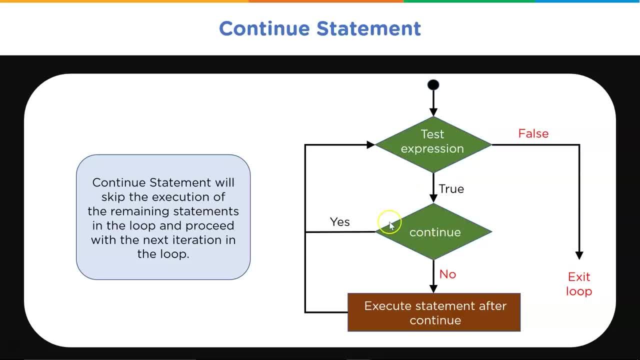 we head to our continuous statement now. if this is yes or true, we again check the test expression. if it is false or no, then we execute the statements after the continuous statement. now we'll understand how the continuous statement works with the help of examples in our demo. 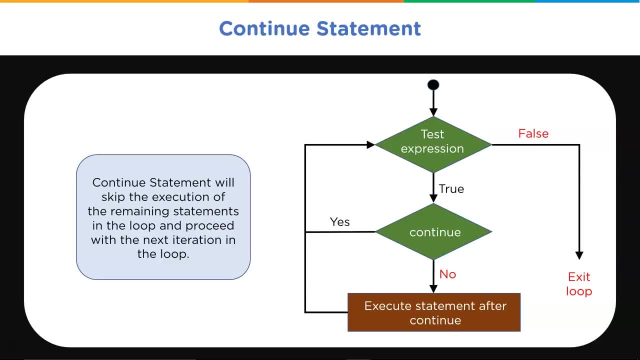 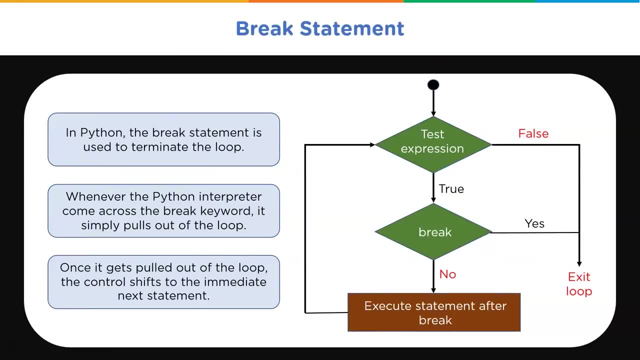 session. so let's see the next statement that we have, which is the break statement. now, in python, the break statement is used to terminate the loop. whenever the python interpreter or the compiler comes across the break statement, it jumps out of the loop, so it skips the remaining. 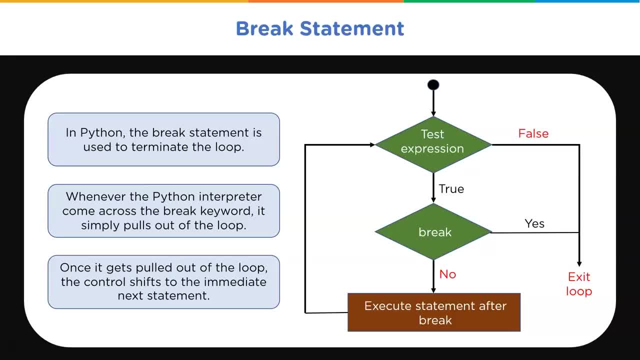 code without further testing the test expression of that loop. now here on the right you can see the flow chart, how the break statement works in python. on the top we have the test expression. now if the test expression evaluates to false, we exit the loop. but but if it is true, then we execute the break statement. if it is yes, then we just exit the. 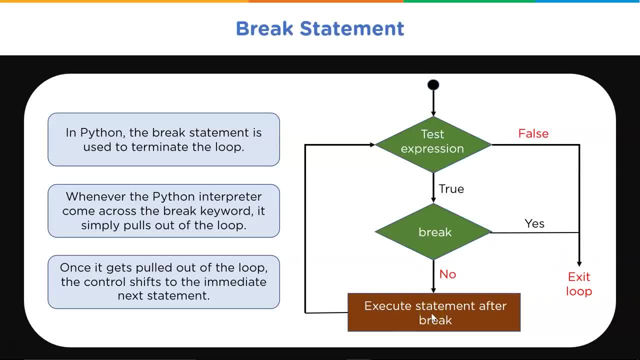 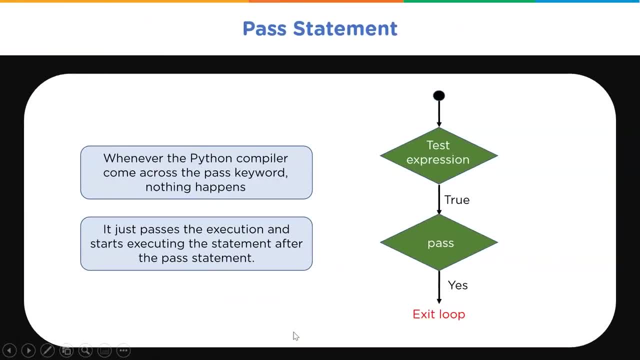 loop. but if it is no, then we execute the remaining statements after the break statement. now moving to the final control statement that we have in python, which is the pass statement. so the pass statement in python is used as a placeholder for future implementation of functions, loops etc. when the 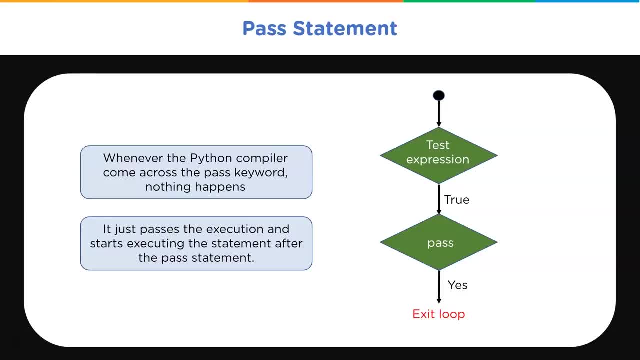 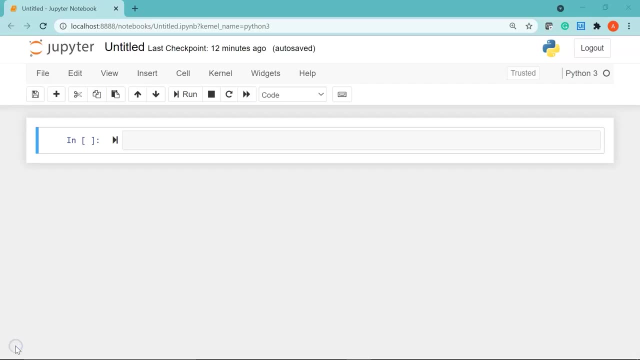 pass statement is executed. nothing happens actually, but you avoid getting an error when an empty code is not allowed. it is also known as a null statement. now let's directly jump to our jupyter notebook, where we'll explore break, continue and pass statements in python in detail. okay, so. 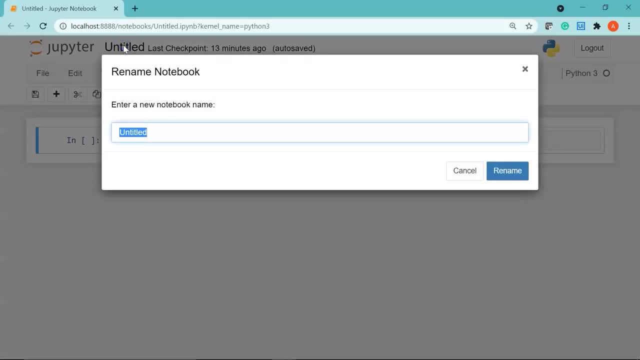 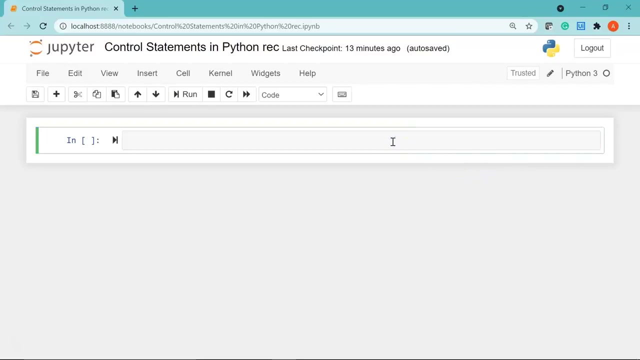 here i am on my jupyter notebook. let me first go ahead and rename my notebook. to control statements in python, i 'll click on rename. okay, now let's see how the continue statement works in python. for that i'm going to print all the letters except the letter i in the string simply loan. so i'll give a comment as: 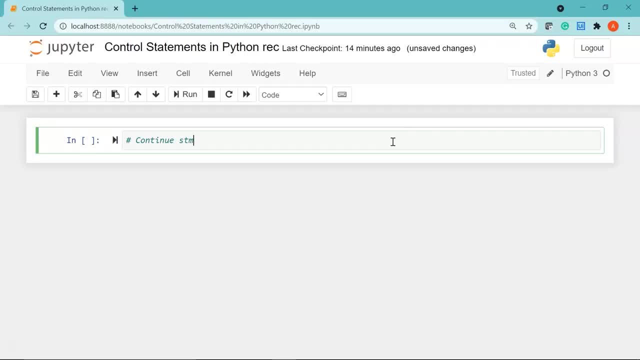 continue statement. okay, so i'll first write my for loop. i'll say: for letters- in my string that is simply loan, give a colon. and then i'll say: if letters is equal to equal to, let's say i, then i'm going to use the continue statement. 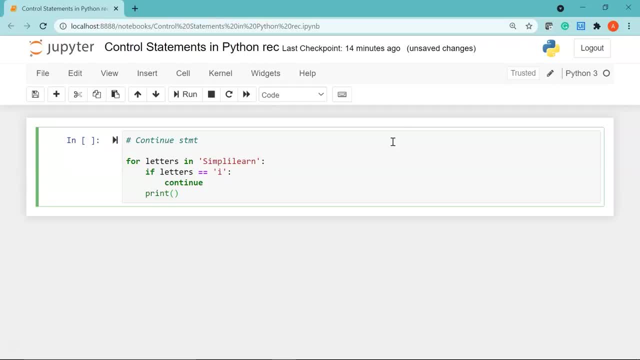 after that i'm going to say print letter. you give a colon, give a comma, and then we are going to print the individual letters in the string. that is simply loan. so here letters is actually the iterator variable. it could be any valid python variable. finally, i'm going to say print- end of execution. 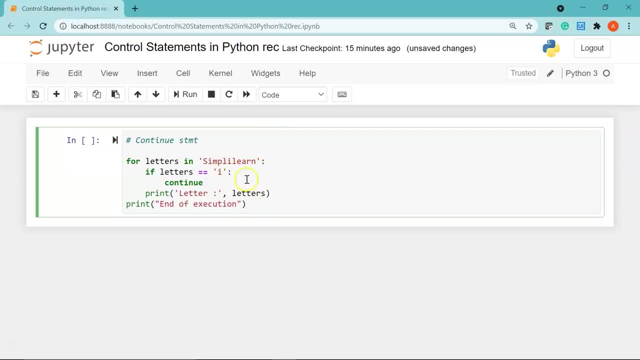 so here, what i am doing is i want to print all the letters except the letter i in my string. simply learn. so whenever the i occurs in my string, simply learn, we'll use the continue keyword and then move on to the next letter in the string. simply learn: if i hit shift, enter you. 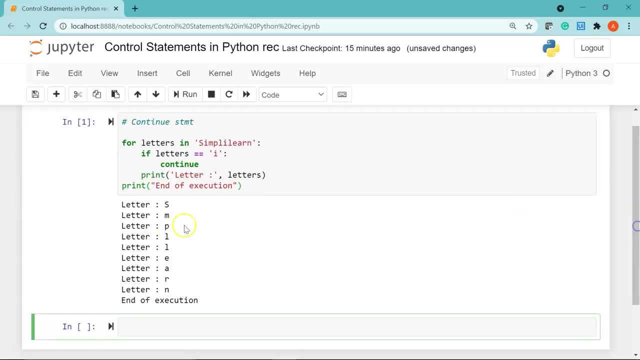 can see the result there. you go here. you can see we have s and the next word was i. so we skipped that iteration, and then we continued with the next iteration. so we have m, p, l, and again here we had another i present in the string. so we skipped this iteration as well and moved on with the next. 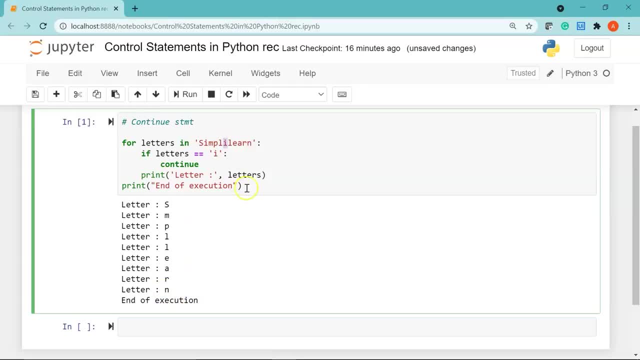 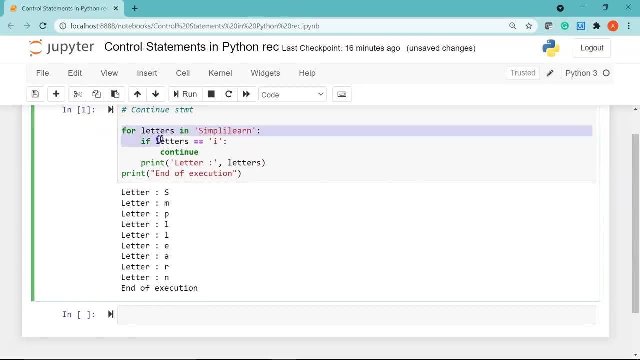 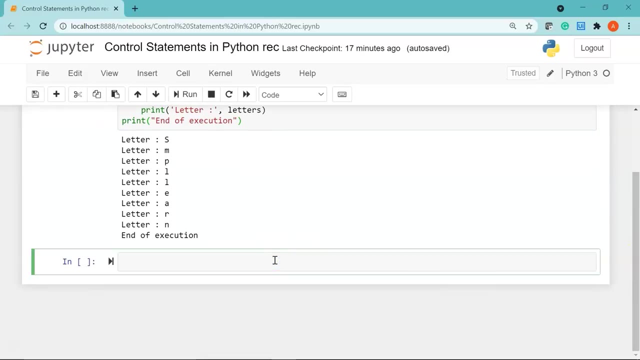 so l, e, a, r and n. finally, we have printed end of execution. so this is how the continue statement works. you can use it in a for loop or you can use it in a while loop as well. now let's see another example where we are going to display only odd numbers present in a list of numbers. so i'll say for: 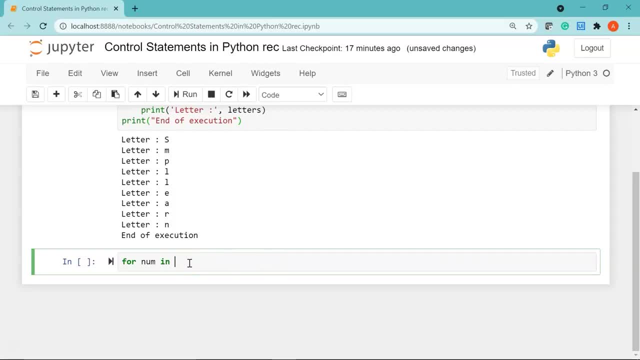 num, which is my iterator variable, i'll say, for num in my list, which has a few numbers, let's say 10, 7, i have 17, let's say 42, 33, 19 and let's say 60.. okay, so for num, my list, which is this one, i'll say: if num mod 2 is equal to equal to 0, so if the remainder is 0, 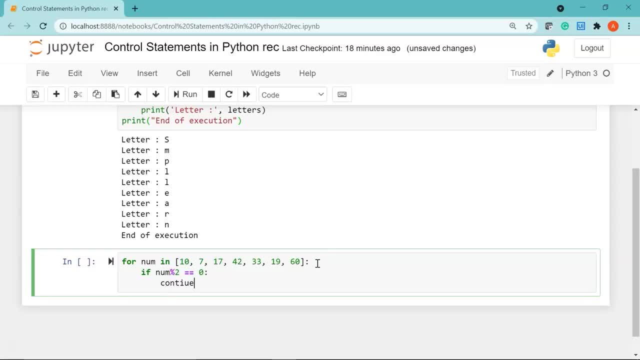 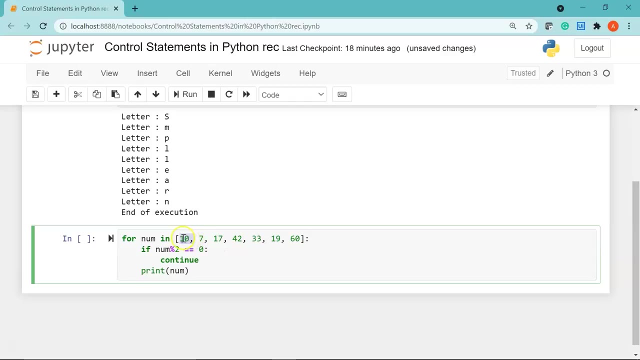 i'll say continue and then we are going to print num. so what we are doing here is, for each number or each item in my list which has a list of numbers, i'm going to check if that number is divisible by 2 or not. if it is divisible by 2, we are going to skip that iteration and we are going. 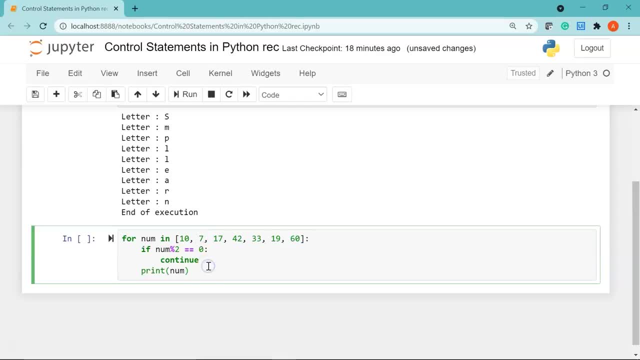 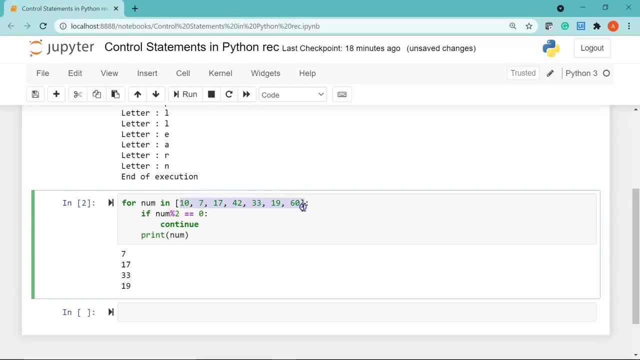 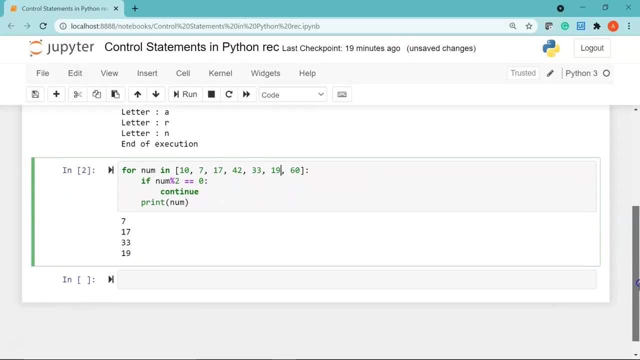 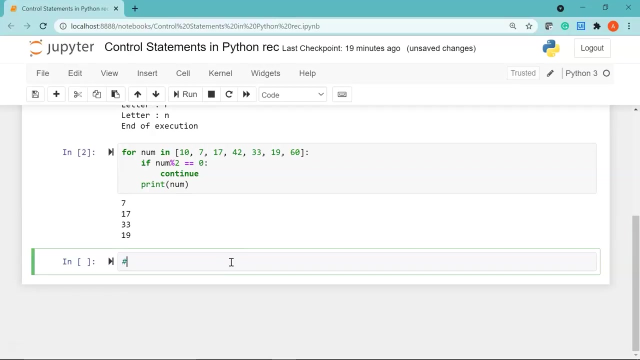 to move ahead with the next number. so let's run it. okay, here you can see we have printed or displayed all the odd numbers that were present in my list, which is this one. so this was another simple example of using a continuous statement in python. now let's move on to the next control statement, which is break. again we are. 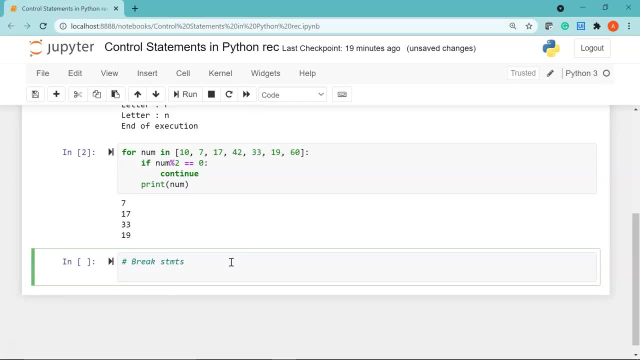 going to look at a few examples here, all right now. the first example we are going to see is how to break the execution when the number 5 comes up in the tuple. so for that we are going to use a while loop. now, first of all, let me declare a tuple. 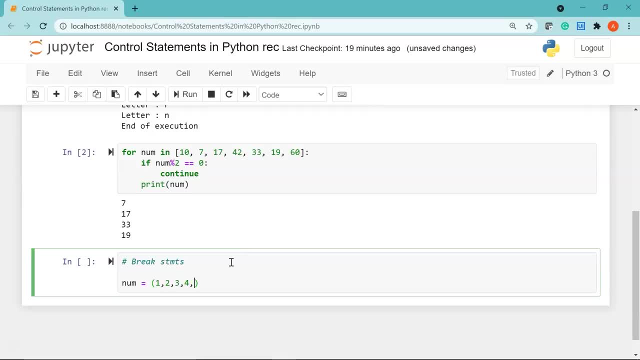 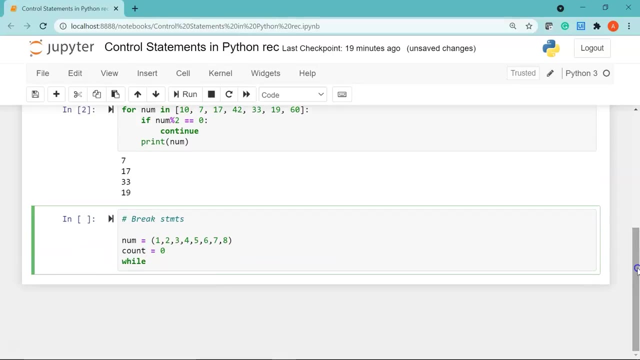 which has, let's say, one, two, three, four, five, six, seven and eight, so numbers from one till eight. i'm going to say count equal to zero and then i'm going to use a while loop. i'll say: while my count is less than nine, then i'm going to write my print statement, print my tuple, which is num, and using square brackets, 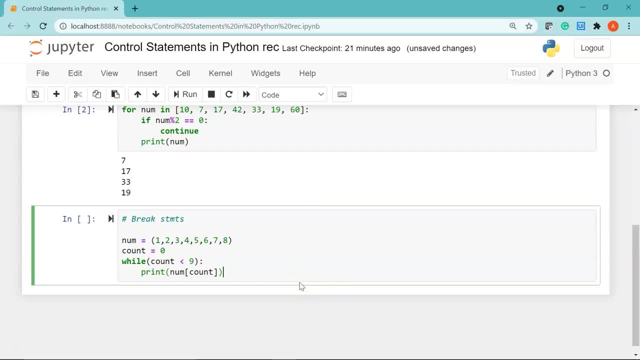 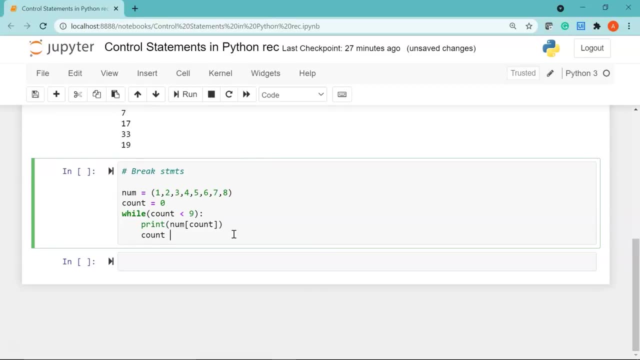 i'll say count. now we are going to increment count by one. so i'll say: count equal to count plus one, and then i'm going to write my tuple, which is num, and then i'm going to write my tuple, which is num. next we will check. if the value of count is equal to equal to five, i'll give a colon. 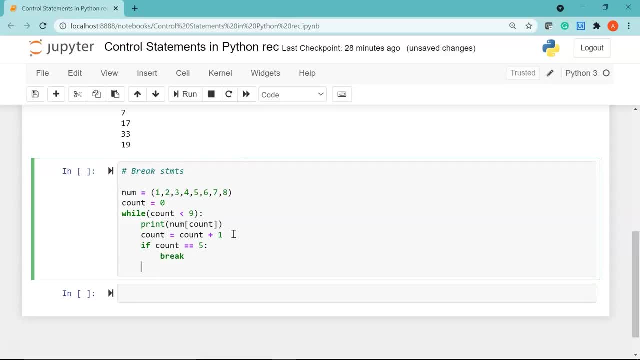 and then we are going to break out of the loop. finally, we'll print end of execution. okay, so this code will help break the execution when the number five comes up in the tuple, which is num. so this code will help break the execution when the number five comes up in the tuple, which is num. 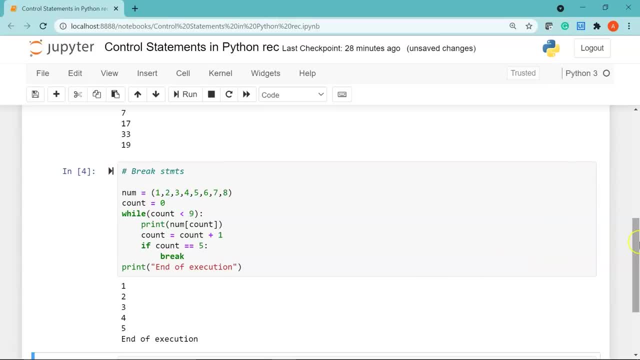 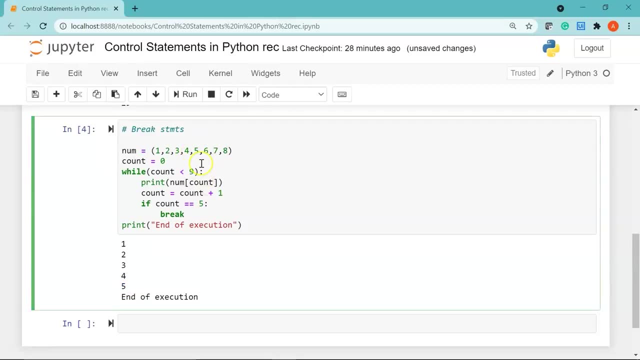 so let's run it okay. so here you can see: as soon as the number five occurred in the tuple, we broke out of the loop and the break statement terminated the execution of the loop. so you can see here: we did not print six, seven and eight and finally we printed our. 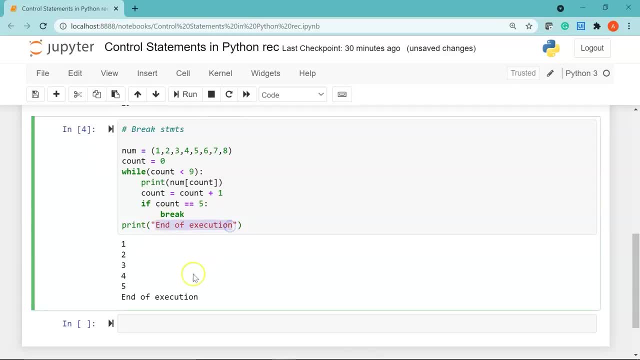 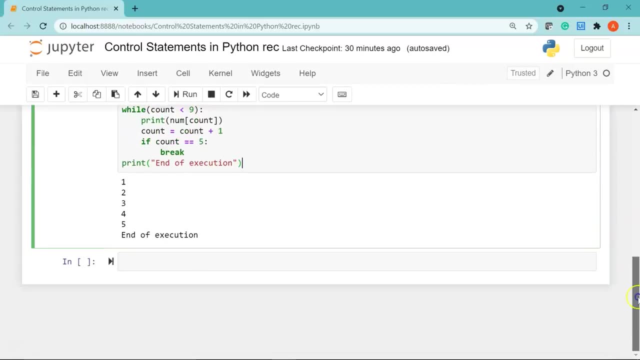 last statement which was present after the break statement. that is end of execution. okay, so i hope this helped you understand how the break statement works in python. we're also going to see another example now. so this is using a for loop, so we are going to break and terminate the execution when. 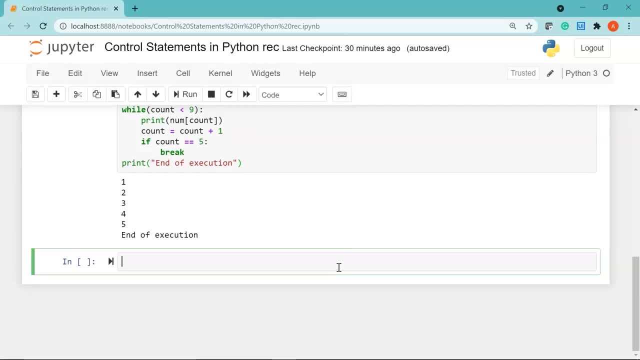 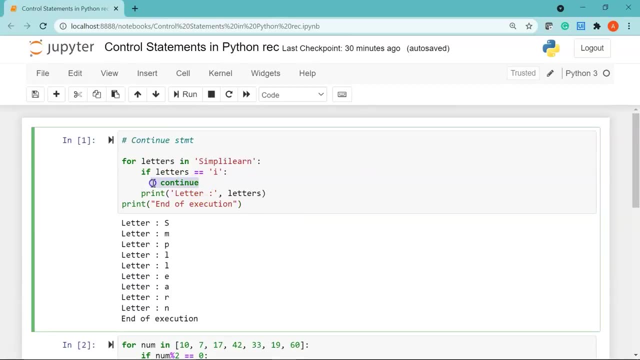 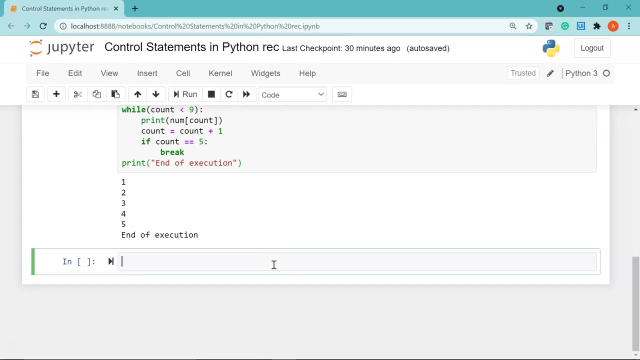 the letter p occurs in the string simply loan. so earlier we had seen one example, which was our first example, where we saw how to use continuous statement for the same string: simply loan. this time we are going to use the break statement to terminate the execution when the letter p occurs in the string simply loan. so i'll start. 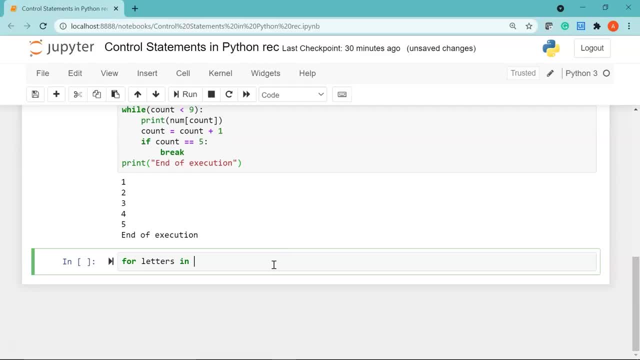 with the for loop. i'll say: for letters in my string, which is simply loan, i'll give a colon and then i'll say: print my message, that is letter. give another colon, i'll give a comma and i'll put my iterator variable, which is letters. then i'll say: if letters equal to equal to. 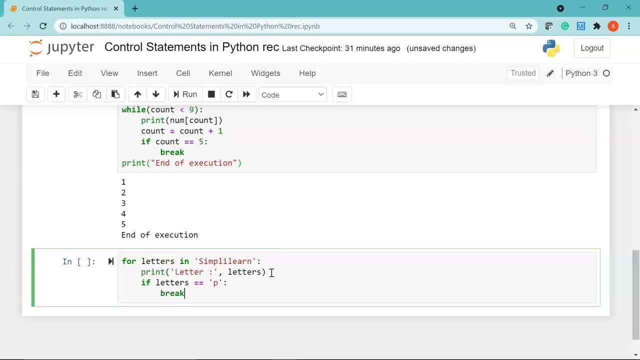 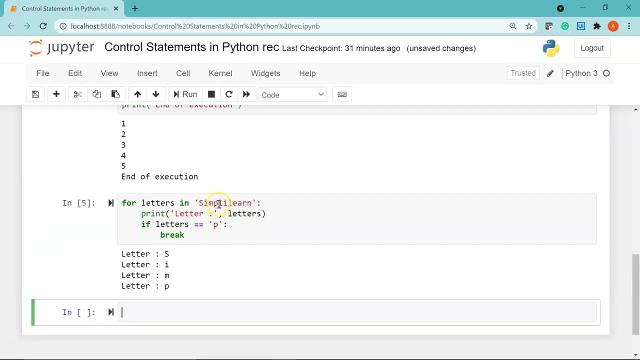 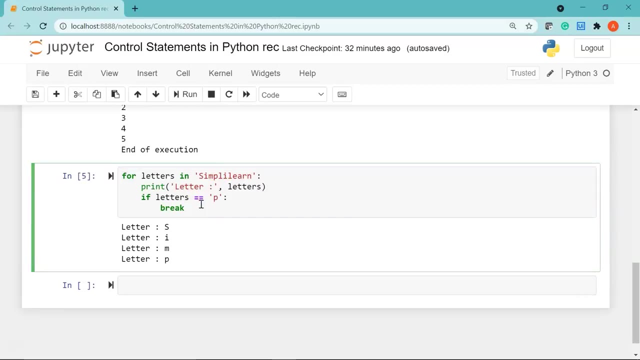 you give a colon and then i want to break out of the loop. now let me just print it. you can see here: as soon as the letter p occurred in the iteration, we came out of the loop. so the break statement executed the above lines of code and the moment is saw the letter P. it just terminated the loop and hence 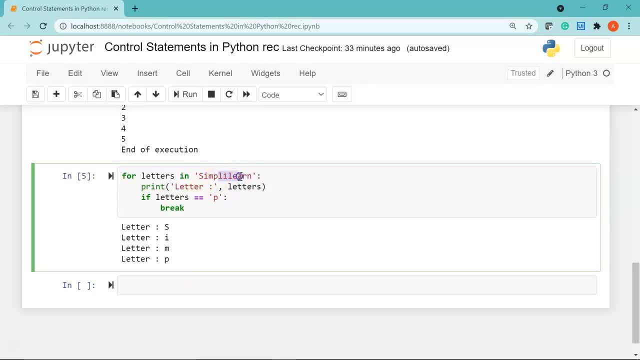 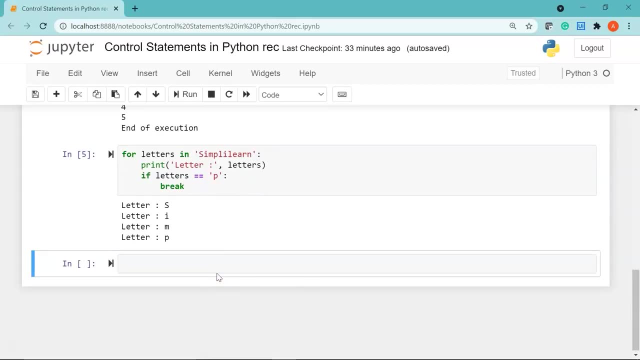 you can see, we did not print the remaining letters in the string. simply learn. okay, now moving to our final section of the demo, where we'll see how to use pass statements in Python. so the first example we are going to see under pass statement is to check if the number is odd. so the number is odd, we are going. 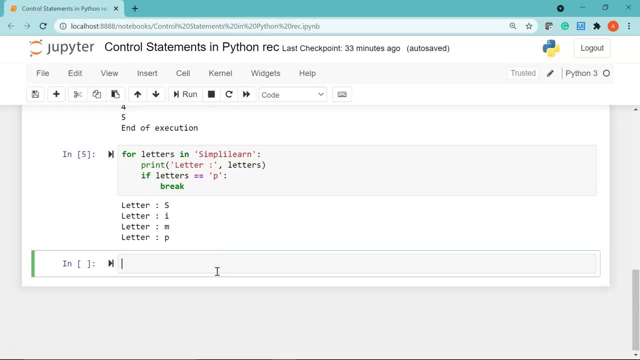 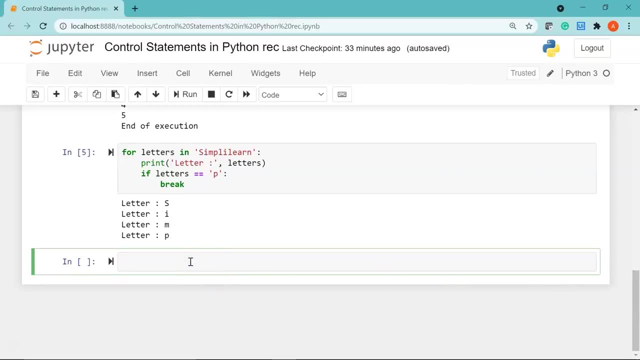 to pass it, else we are going to print only the even numbers. okay, so for that I'm going to use a for loop. but before that let me just give a comment. I'll say pass statement. okay, so in the first example we'll check. if the number is odd, then we are going. 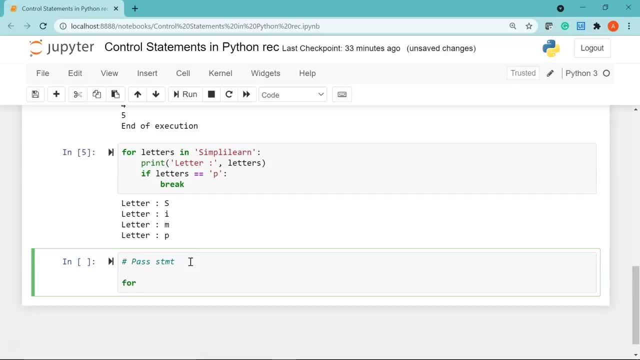 to pass it and only print the even numbers. so for that I'm going to use a for loop. I'll say for number in range. let's say I'm taking the range between 10 and 25. give a colon. I'll say if number mod 2. 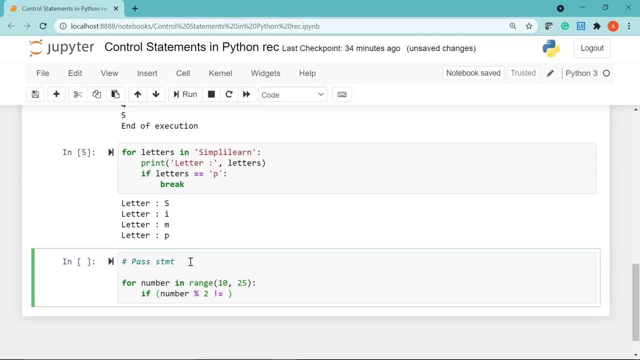 if it is not equal to 0, give a colon, then we are going to pass it. so this means if the number is odd, then just pass it, else I'll say print the number is, give a colon, the comma, and then I will pass in my iterator variable which. 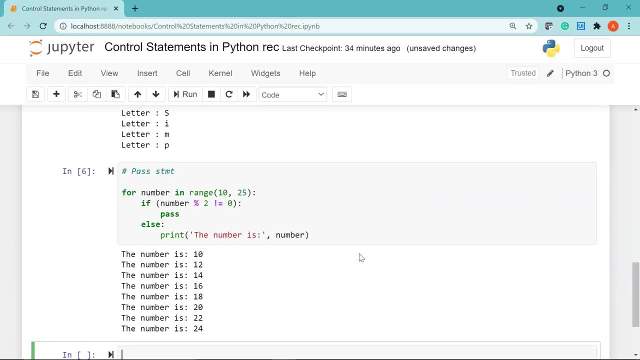 is number. now let's run it. okay, you can see here in the range 10 and 25 we have excluded all the odd numbers because we use the pass statement. so it passed printing all the odd numbers and it just printed whatever those there in the else. 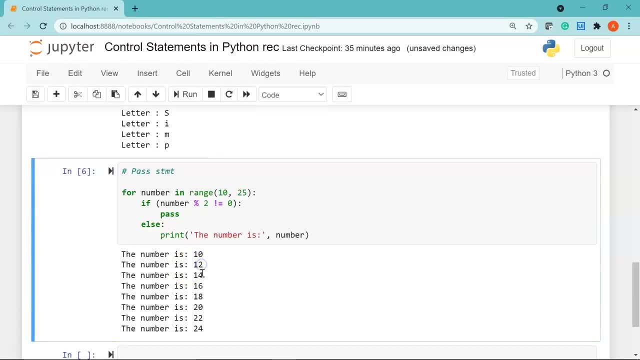 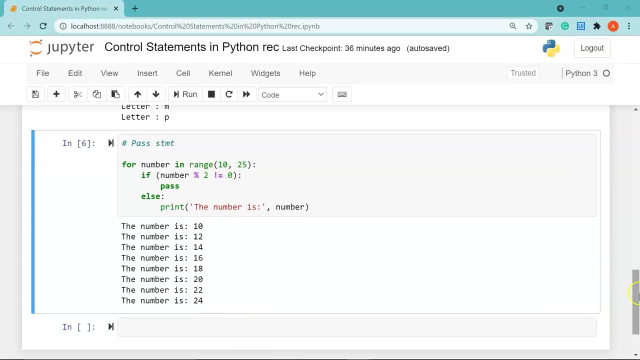 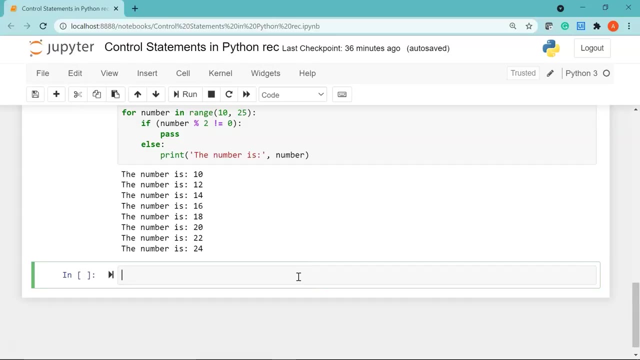 part. that is the even numbers. we have 10, 12, 14, then we have 20, 22 and 24. so these are all the even numbers that lie between 10 and 25. all right now coming to the final demo. so here I am going to write a user defined function to print. 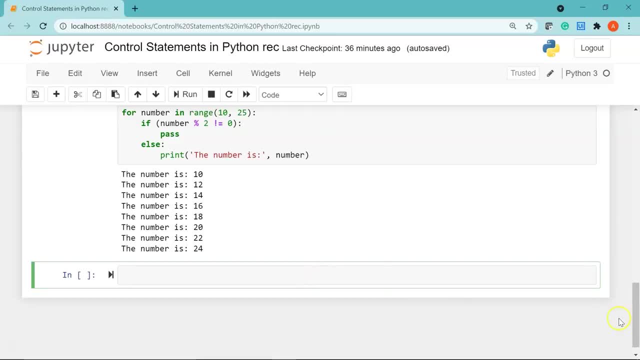 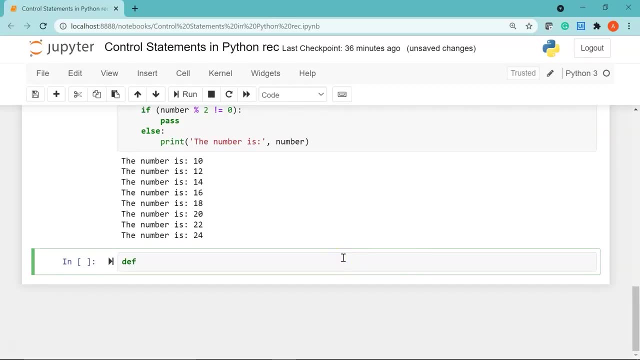 any number other than 10. so again, we are going to use a pass statement for this. so let me write my user defined function. I'll use the def keyword and my function name. let's say: print underscore num. then I'll pass in my parameter. let's say: 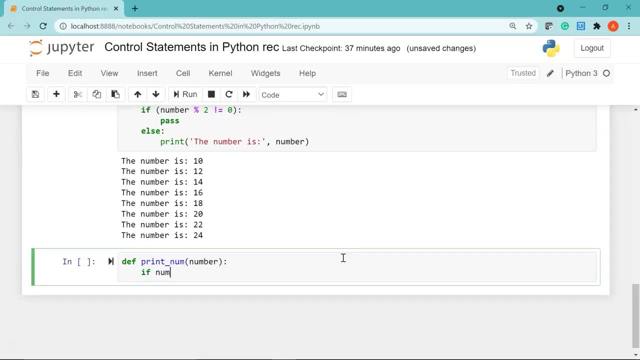 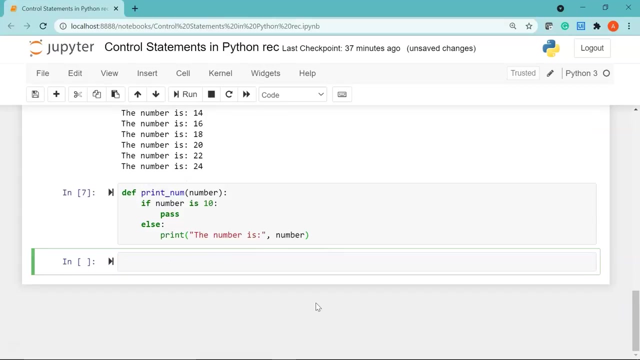 number, I'll say: if number is 10, then I'll use the pass statement. otherwise I will say: else, print the number is. I'll give a comma and then I'll say number, which is there in my parameter. now let's run it now. we are going to call the function using the function. 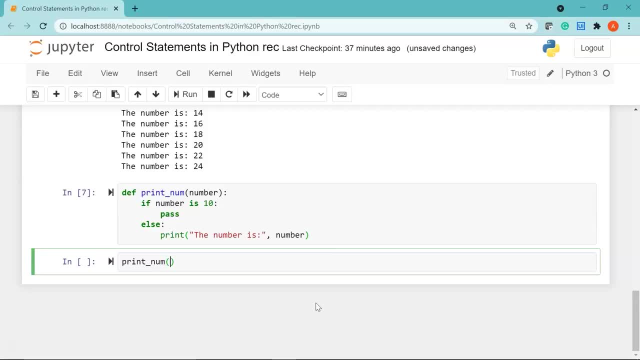 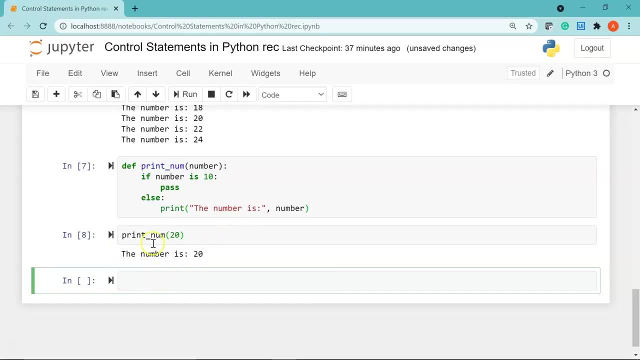 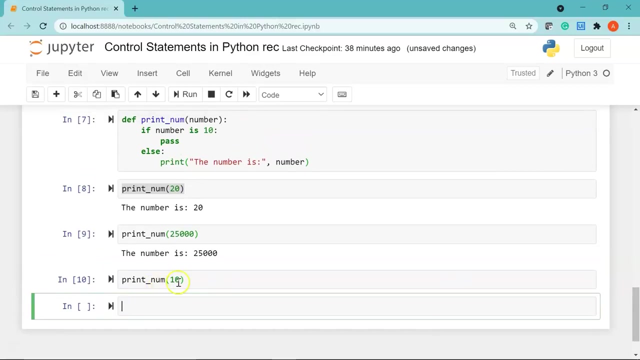 name, which is print num. if I say print num 20, it will print my number saying the number is 20. let's copy this, I'll paste it here. let's say I'll say 25,000, it is going to print 25,000. but if I say print num 10, you can see it here that Python has just passed. 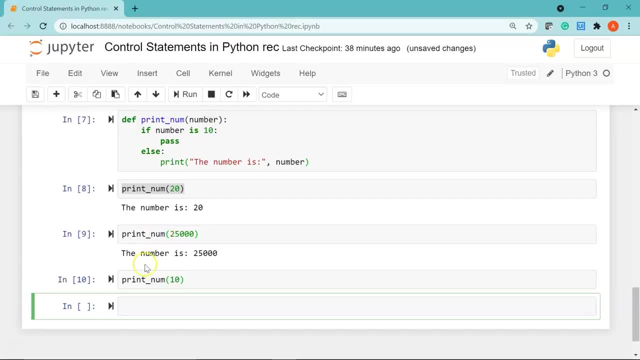 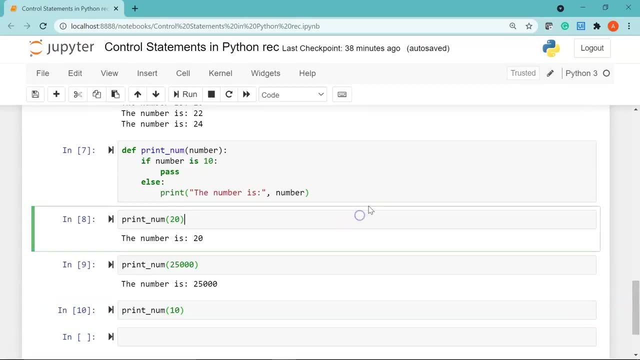 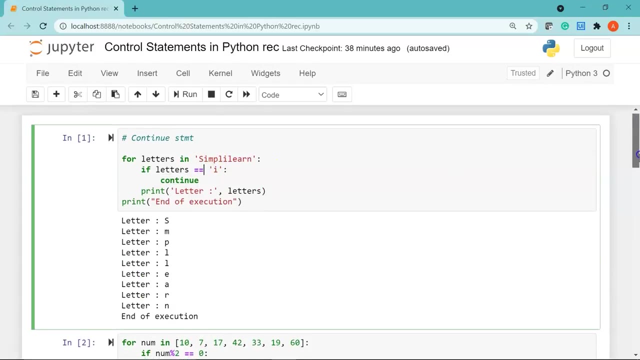 it because we had given in our condition: if number is 10, then just pass it. so there was no output for 10. all right, so that brings us to the end of this demo session on control statement in Python. so we looked at how the continuous statement works. then we saw how the break statement works. we 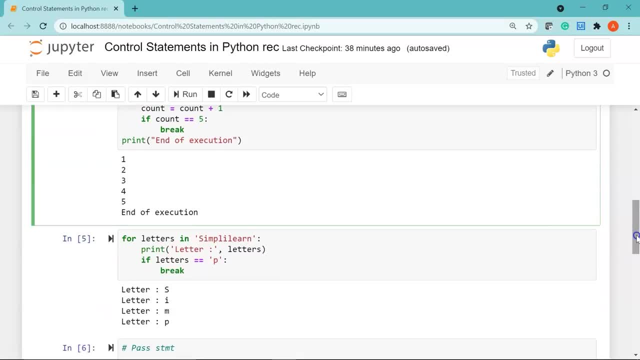 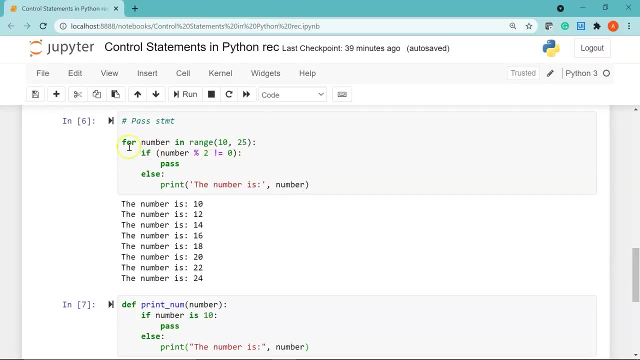 looked at two examples: one was with while loops and the other one was with for loop. and finally, we saw two examples on passed statements. one was using for and if else and the other one was using a user defined function and inside that we used the if-else condition. 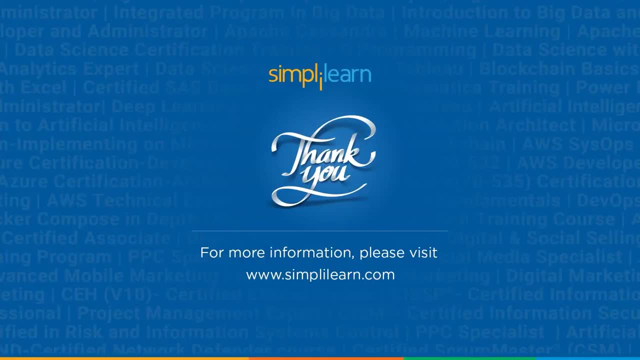 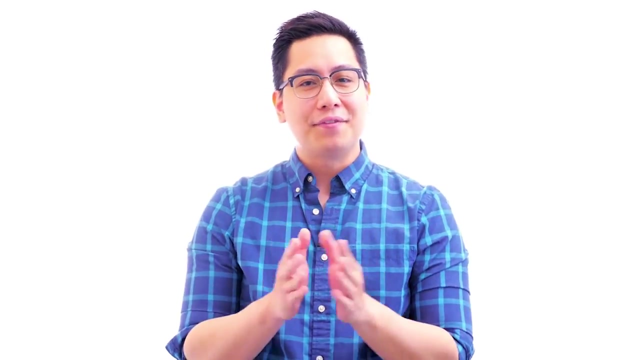 so that brings us to the end of this video tutorial on control flow statements in python. i hope this was useful and informative. if you have any queries, please feel free to put them in the comment section of the video. thank you for watching hi there. if you like this video, subscribe to the simply learn youtube. 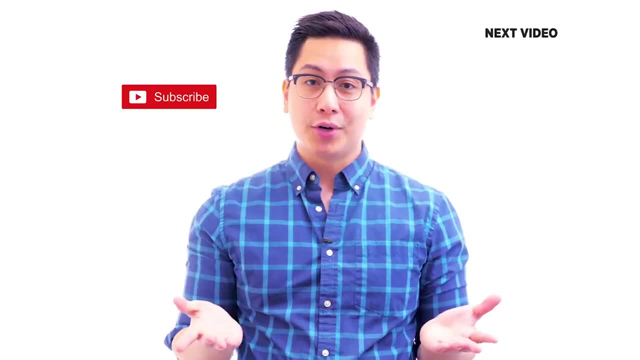 channel and click here to watch similar videos. to nerd up and get certified: click here. 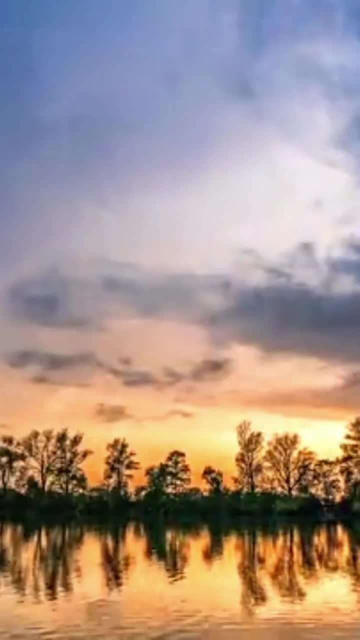 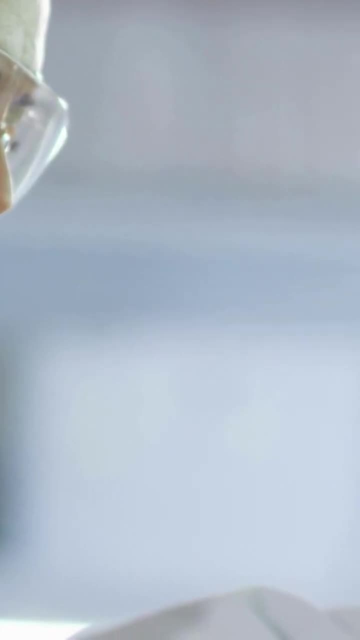 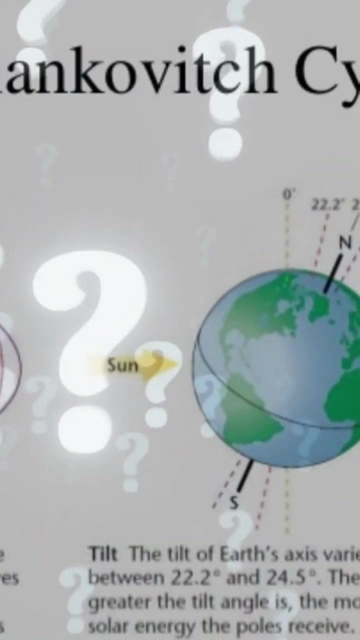 Have you ever wondered why Earth's climate fluctuates between ice ages and warm interglacial periods? Scientists have been trying to answer this question for a long time, and Milankovitch cycles offer an explanation. So what are Milankovitch cycles? 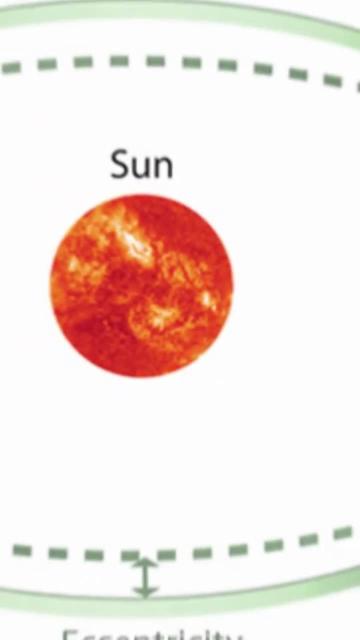 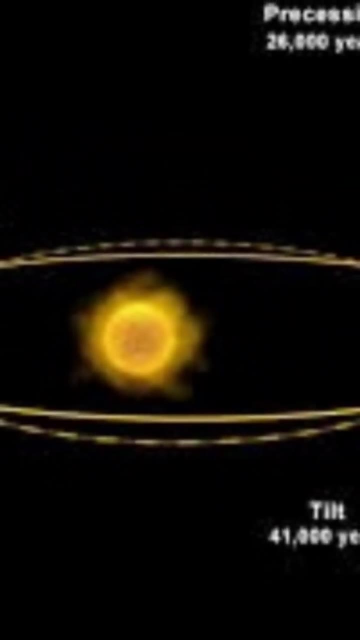 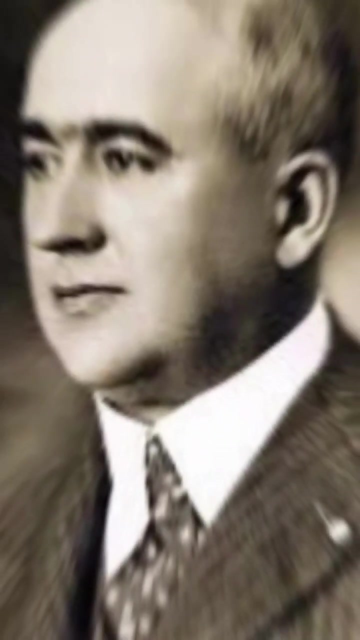 Milankovitch cycles are long-term variations in the Earth's orbit around the Sun. These cycles affect the amount and distribution of solar energy that reaches Earth, which in turn influences the climate. They are named after the Serbian geophysicist and astronomer.